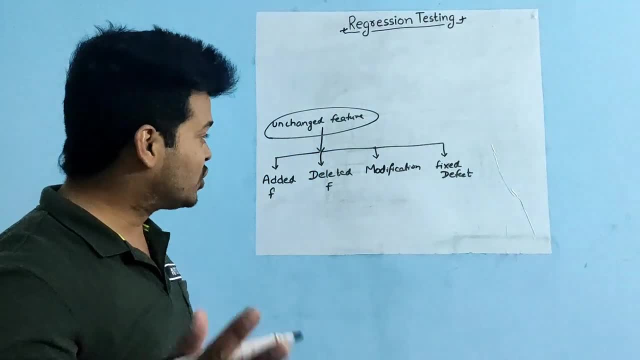 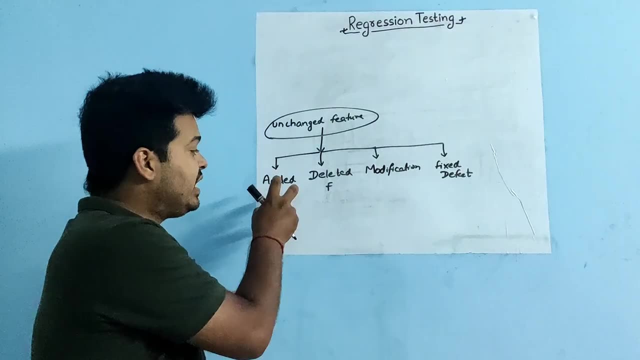 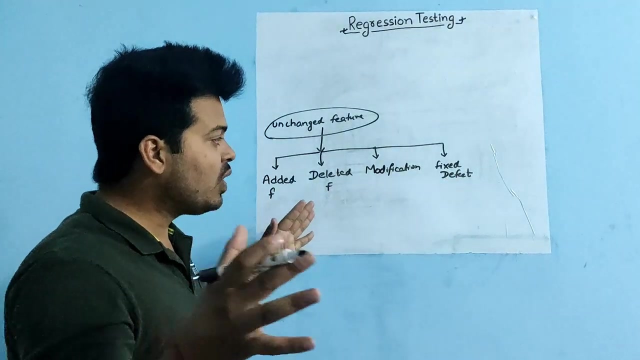 that is called as regression testing. so you test the unchanged feature to make sure that whatever the developer has done he had, he have added some feature, he has deleted some feature, he has done some modification, he has fixed some defect. so you are as a part of regression testing. 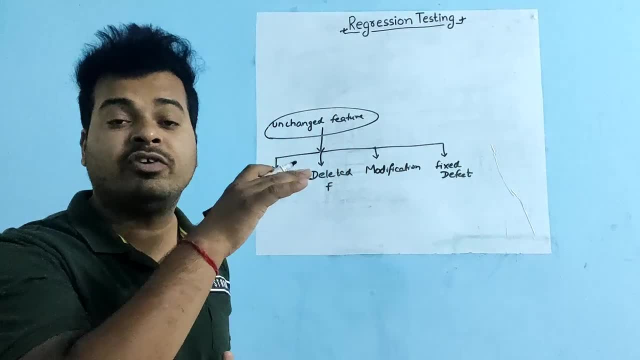 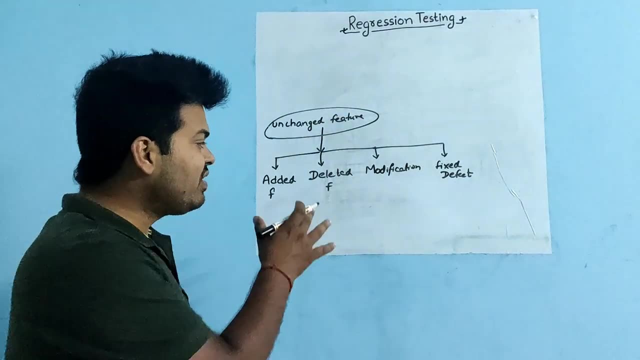 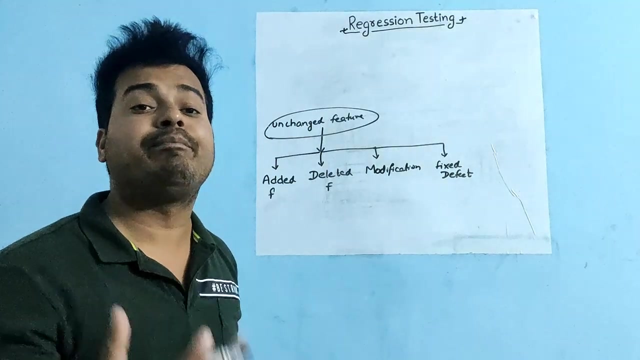 you are testing the unchanged feature, the feature which are not at all changed. you are testing the unchanged feature as a part of regression testing to make sure that, whatever developer has done all these three, four or, because of this four, my unchanged features are not impacted or not. 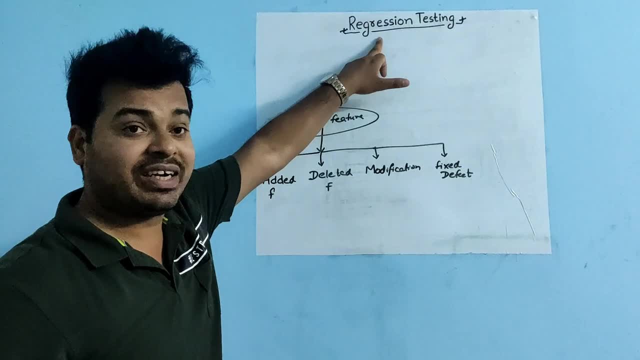 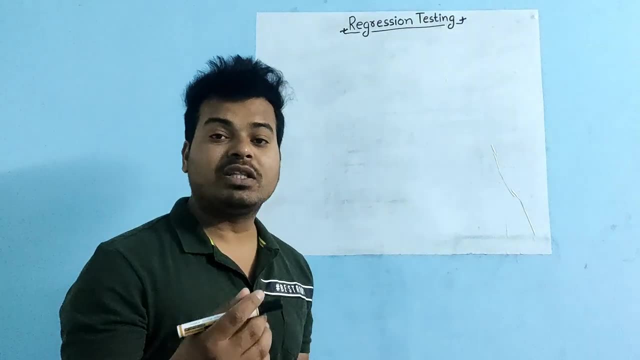 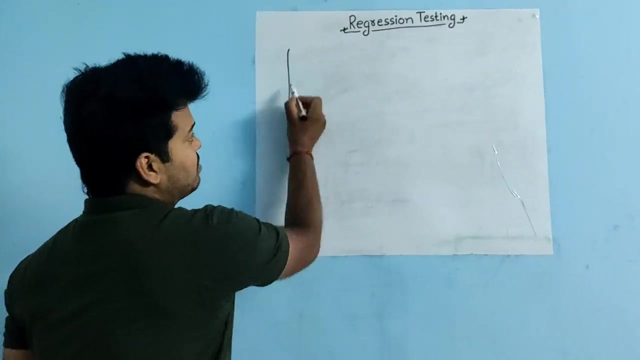 affected. i will make sure that by doing regression testing. now we are going to talk about what are the various types of regression testing. so, depending on the modification or changes done by the developer, the regression testing are classified into three types. first type of regression testing is called shake out as attitude. 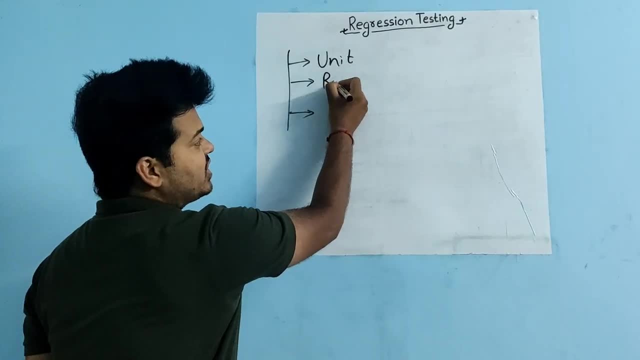 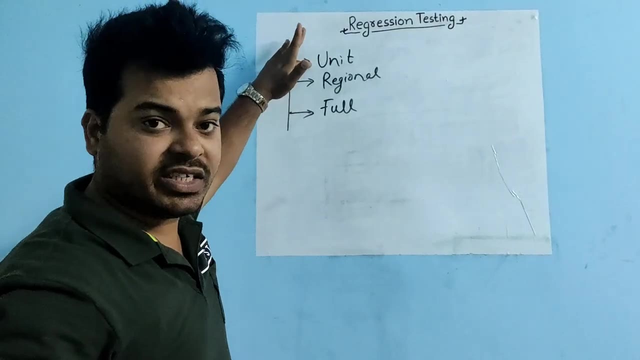 station seems to say that you call that regionalism. just as good time outside the, because interesting is called as fully version destiny. now, what do you mean by education? testing? okay, e, but I liked this. I not liked the idea of values on campus in this point, but I will hope you. Unit regression testing means testing only the changes or modification done by the developer. So unit regression testing is nothing but testing only the changed part or modification part is called as unit regression testing. Suppose you are having an application in which you are having username, password and there is a login button. 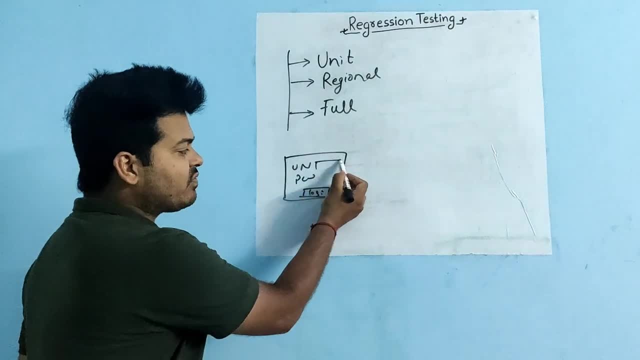 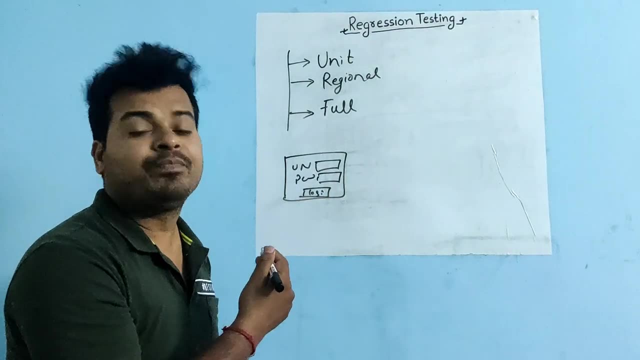 Now developer has done some changes in username text field and password text field, Because of which, when you are entering your username and password and you are clicking on login button, it is not allowing you to proceed to the home page. It is not taking you to the home page. 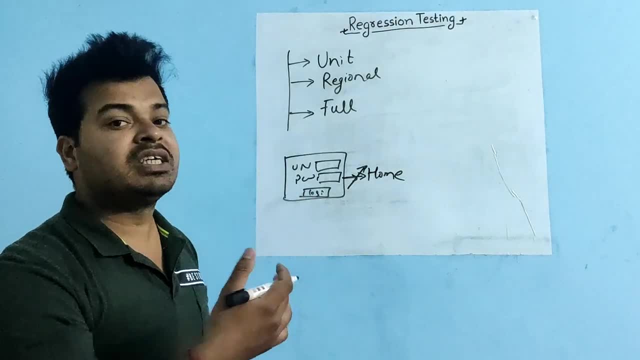 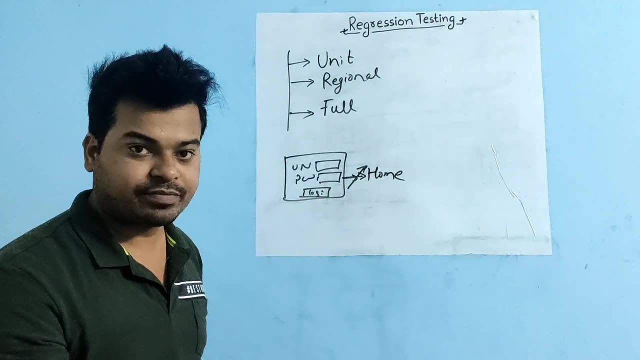 Home page is not coming. When you are clicking on login page, some different thing is coming. It is telling password is not matching, or it is going to the blank page. Let's say it is happening because developer has done some changes in username text field and password text field. 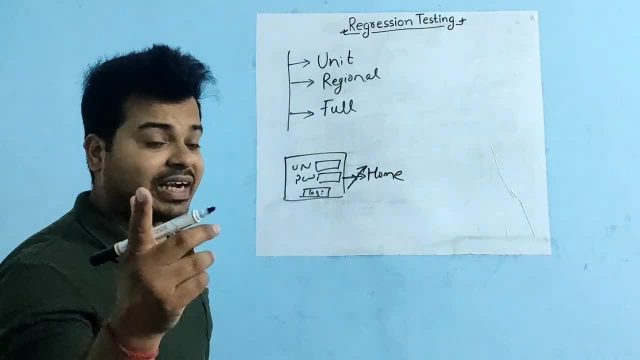 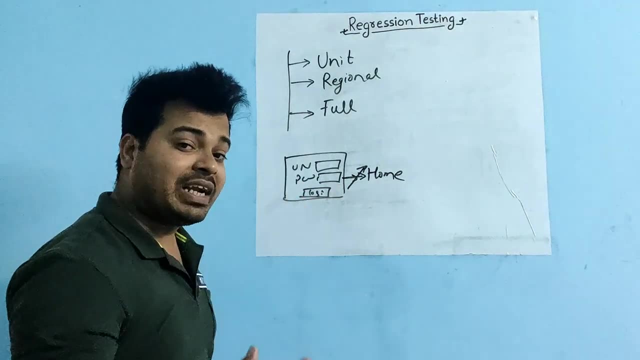 In that case, what you will do- He will give a fix That time- you should do unit regression testing, Testing only the changed part or modification part That is called as unit regression testing. Now, what do you mean by regional regression testing? 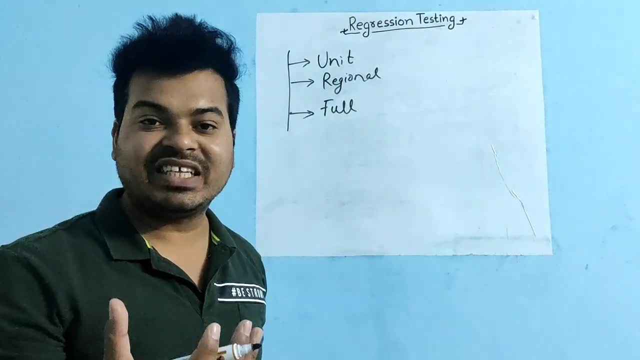 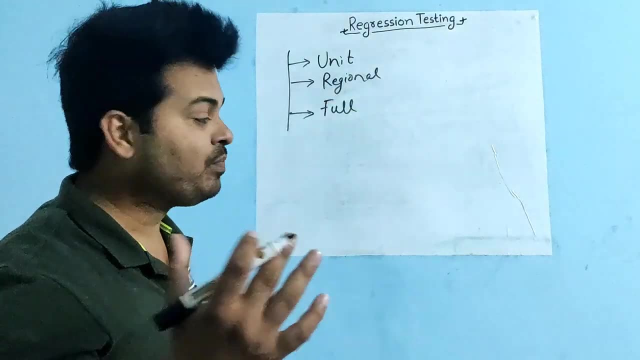 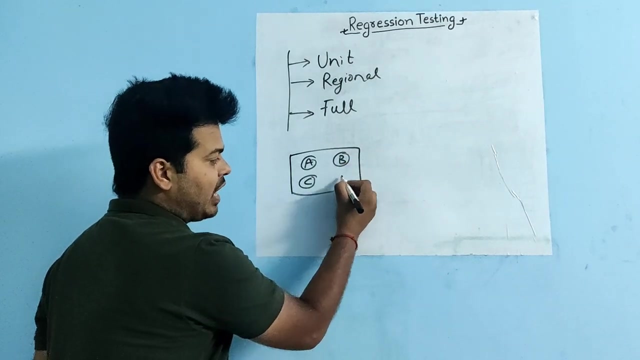 So regional regression test? the definition says that testing the changed part and also the impacted areas, That is called as regional regression testing. Suppose you are having an application which is consisting of four modules: Module A, Module B, Module C and Module D. 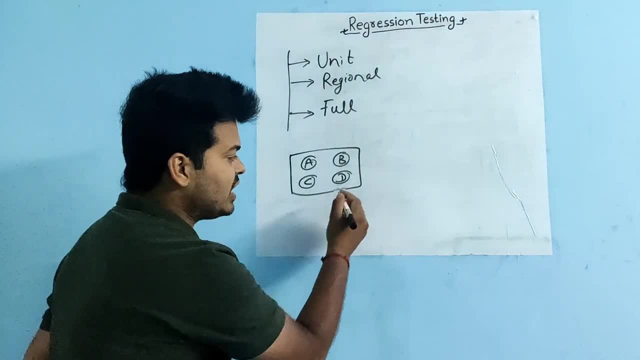 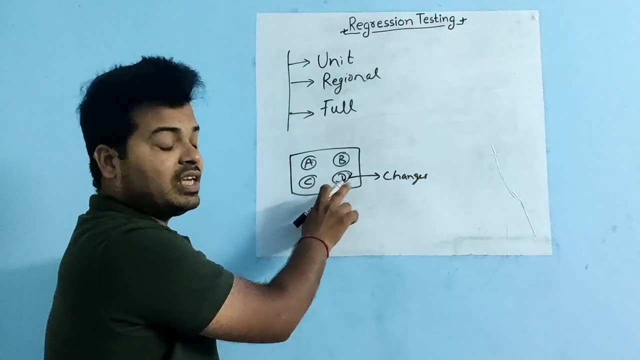 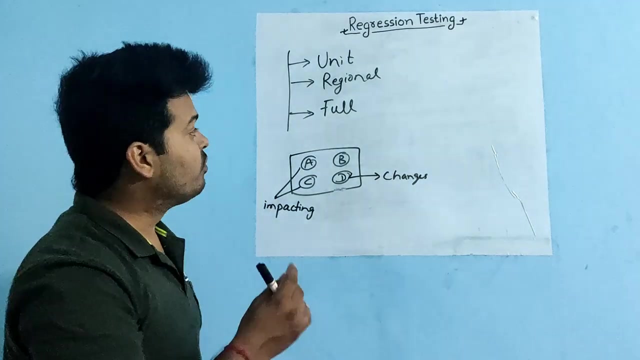 Now, developer has done some changes in module D. Developer has done some changes in module D. Modification done in the module D is affecting my module A and my module C. In that time, what you will do? You will do regional regression testing. You will do testing the changed feature and also impacted areas. that is called as regional regression testing. now the question arises, when you are testing the application, how you will get to know that which is my impacted areas, which which all are my impacted modules. so, before proceeding to the 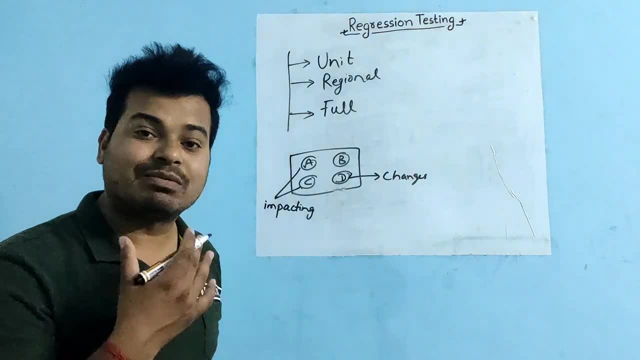 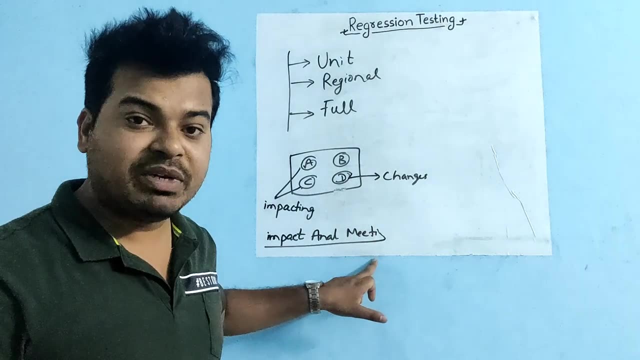 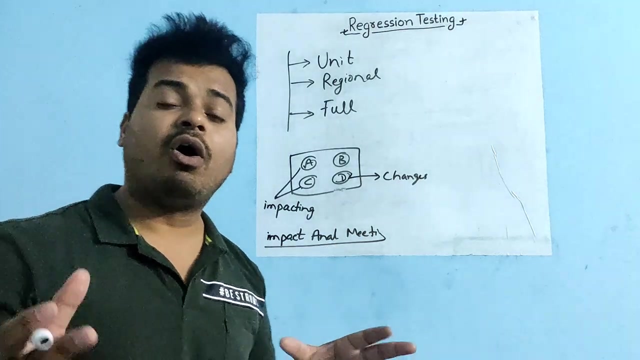 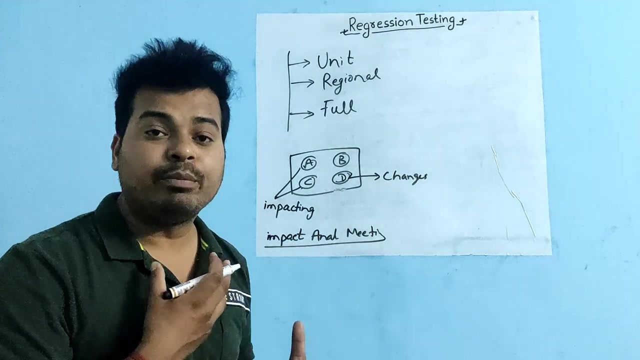 testing. there is a meeting which is called as impact analysis meeting. there will be meeting called as impact analysis meeting. impact analysis meeting is a meeting conducted by the test engineer or business analyst or product manager in which all developer, test engineers and my product manager will sit together and they will decide if I am doing some, if developer is doing some. 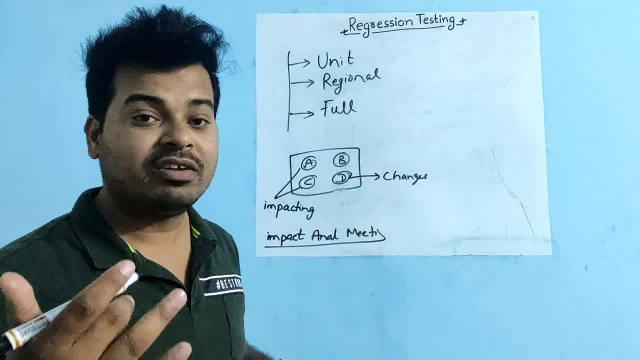 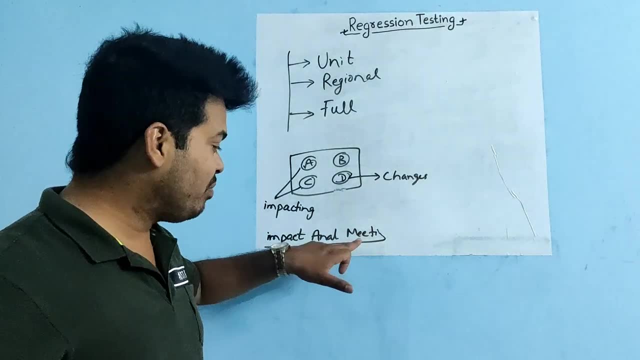 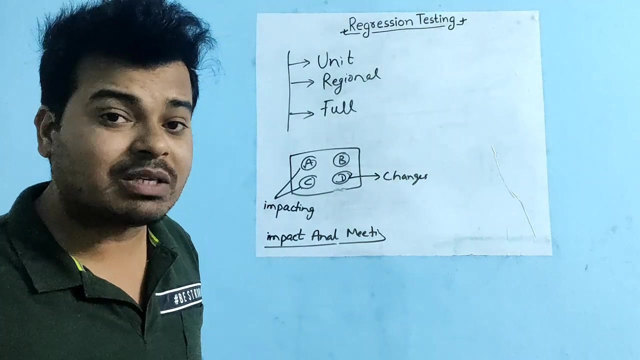 changes in my module, see which and all feature it can affect which and all module can affect. so impact analysis meeting. so by doing impact analysis meeting, QA or tester will have a meeting. so by doing impact analysis meeting, QA or tester will have a correct understanding that if my developer is doing some changes in 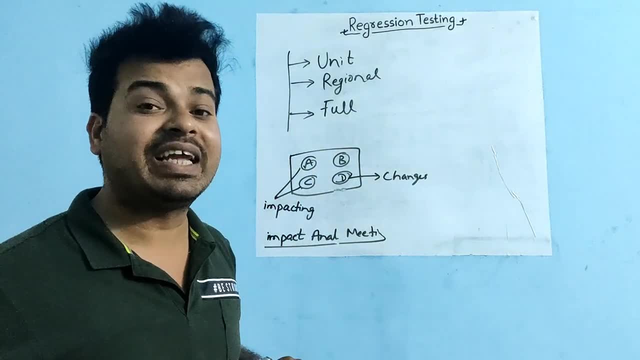 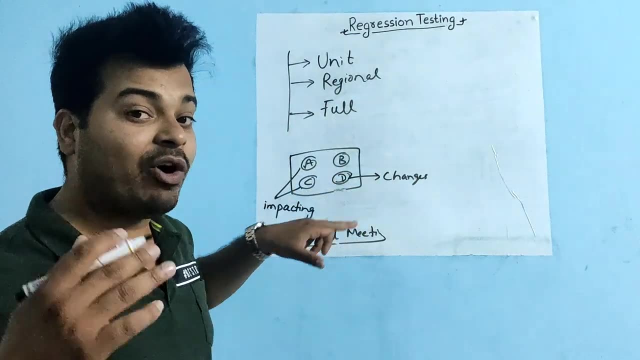 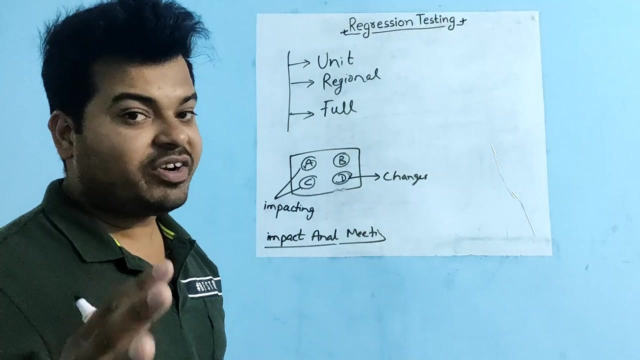 module D, which all modules will get affected. so, as I said, regional regression testing is nothing but testing the changed part and also the impacted part. it is called as the regional regression testing. now you will talk about what do you mean by full regression testing. so full regression testing is nothing but. 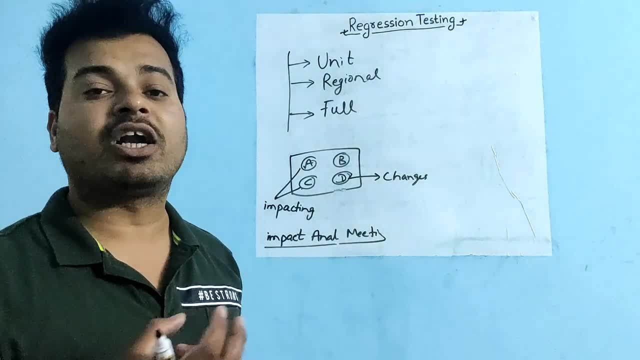 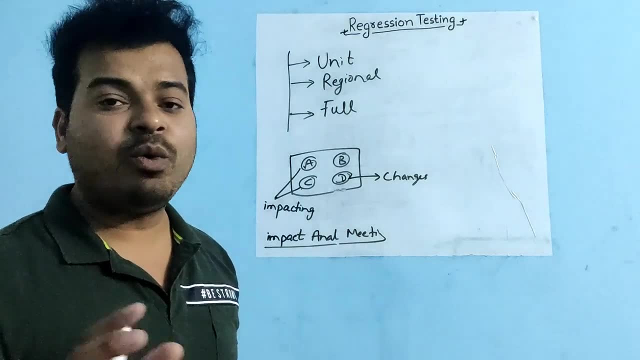 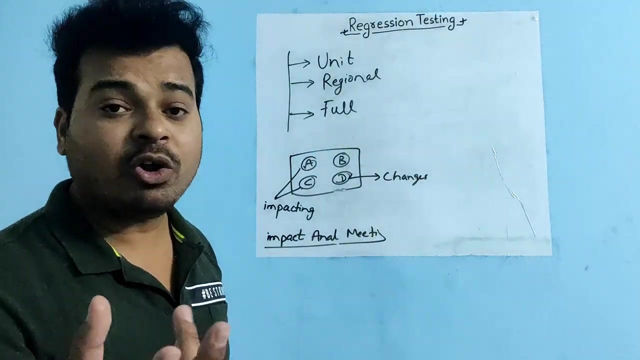 testing the change feature and also the remaining part of the application. it is called as full regression testing. so as a part of full regression testing, no matter where developer has done the changes, if you are doing full regression testing, that means you have to test not only the change part but all the remaining part. 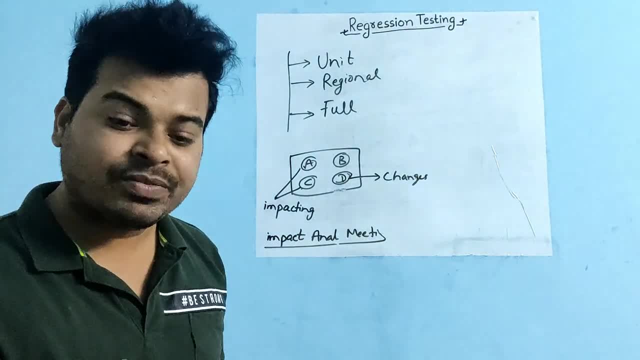 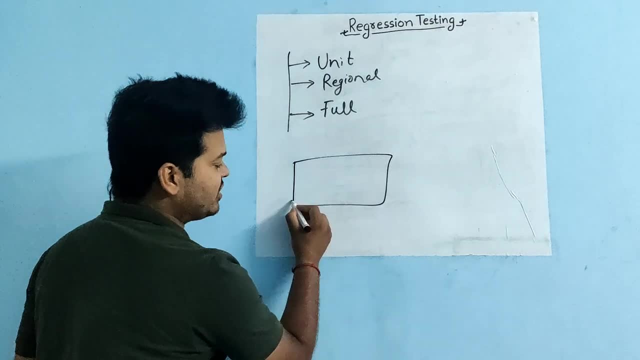 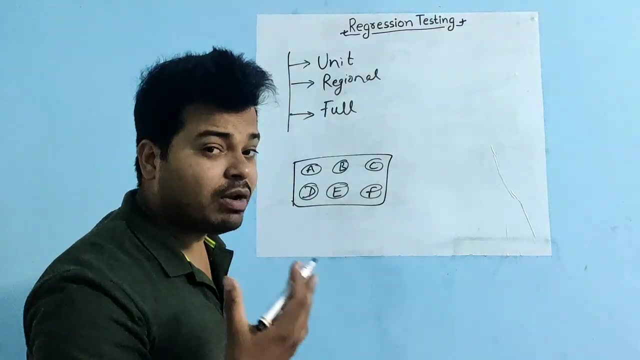 of the application. that means you have to test the change feature and also all features present in the application. suppose you are having an application in which you have a faults in it or any defects of the application. one change, even if not. there is also a ludicrous change. Lord said: hey, developer, did change in it and change points too. but 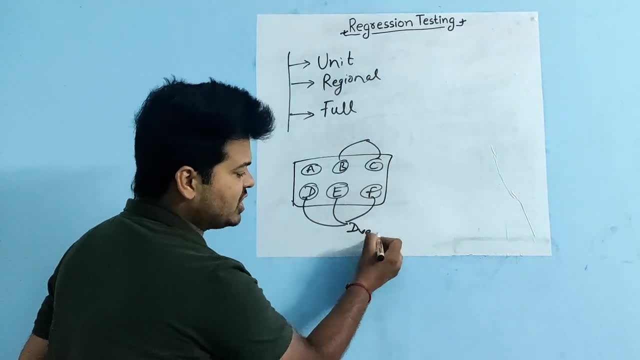 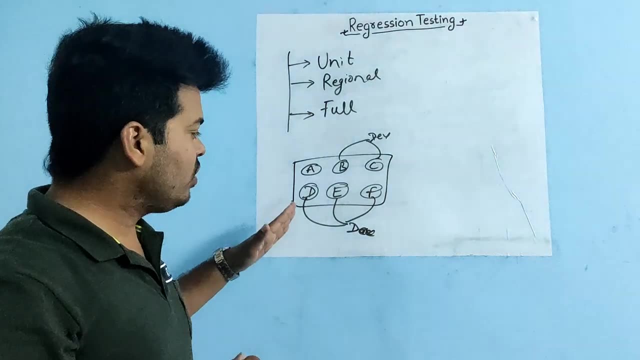 there are some other changes. it is not like if developer changed module A to module B, to module C, to module B to module C, to the to E development. a developer changed through the module A. the change that is carried out over the development there had a culprit. I did not have any changes in module D, module E, module F. Developer is: 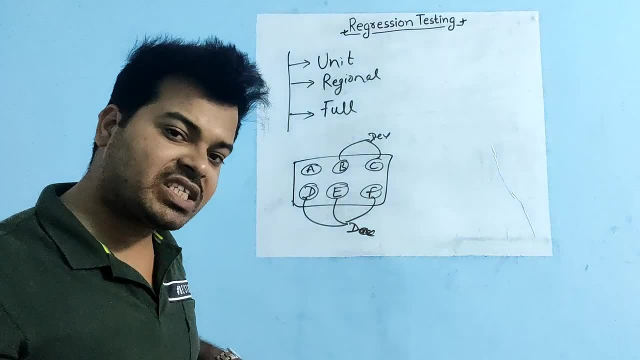 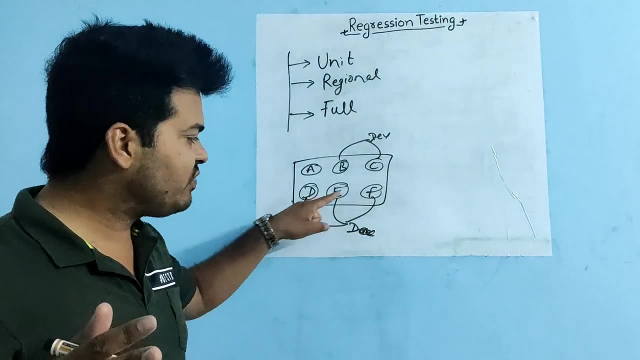 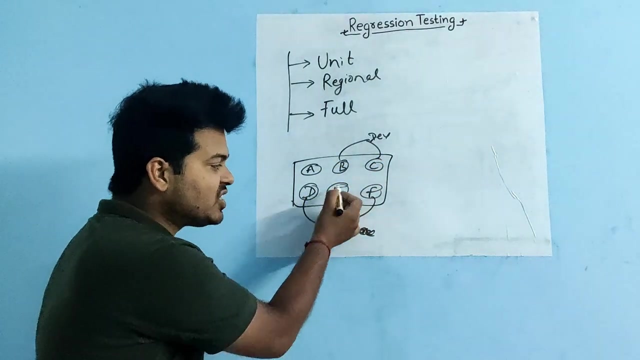 done now, changes in module B, C, E, F, D. now developer has done some changes in this modules. finally, what you will do: not only the change feature, but you will also test all the remaining modules present in application. you will test not only the change feature, but also all the feature present in the application. what 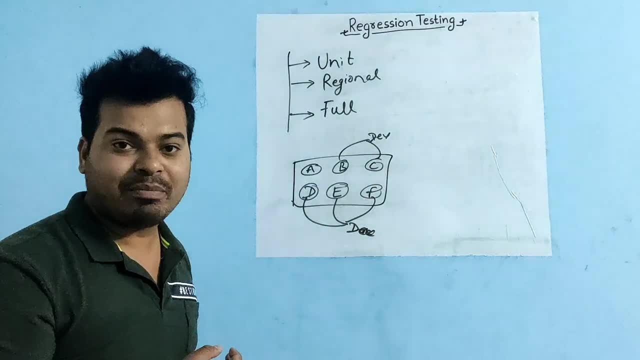 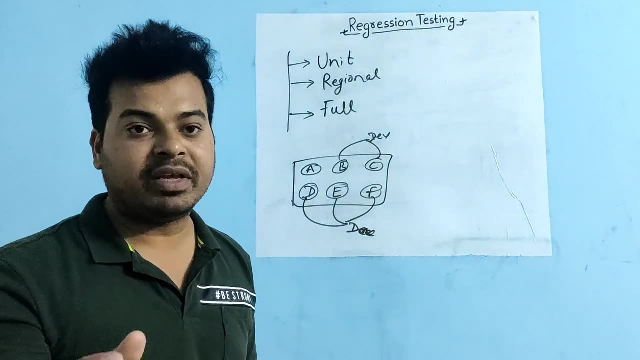 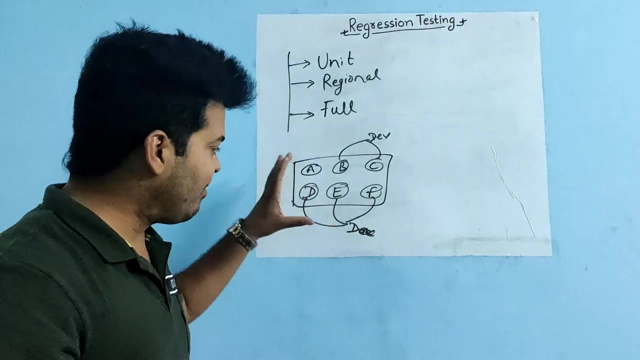 is the reason behind that why you will test all the remaining feature of an application. because if developer are doing some changes in most of the module, don't waste time in finding out which you know are the impacted areas. it is a waste of suppose you are having a more if you are having an application in 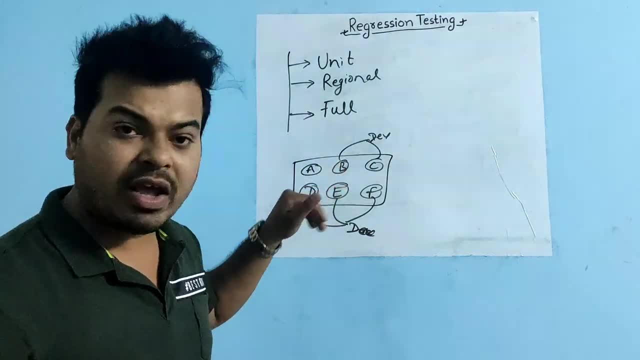 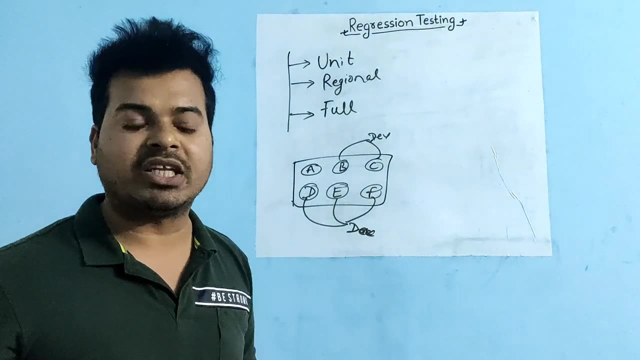 which there are six modules and developer has done changes for five modules or four modules. if you try to make a impact analysis meeting, you will call business analyst or product manager or developers or QA. then you will have a meeting of one hour and you will decide which in all modules if we have done. 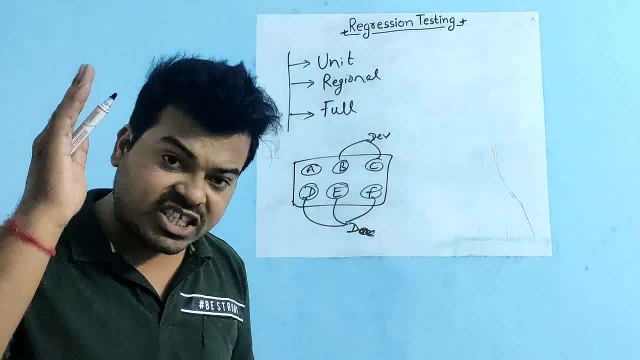 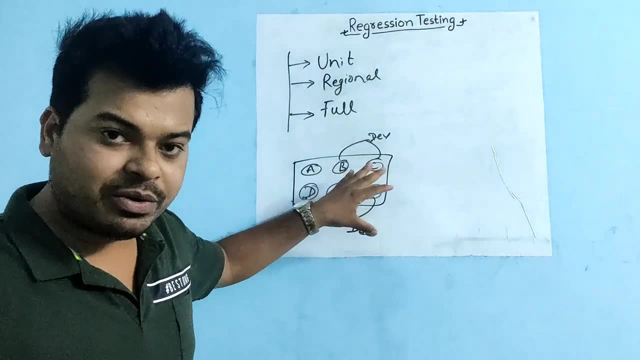 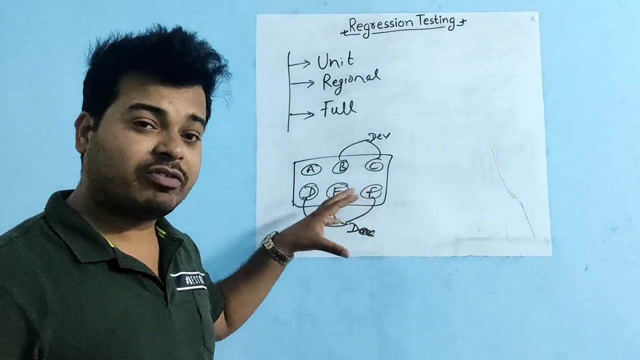 changes and this module, which, in all modules, are getting affected. instead of that, instead of wasting this time, since developer has done the changes in most of my module in my application, it is preferable that when developer has done changes for most part of the application, it is highly preferable to do full. 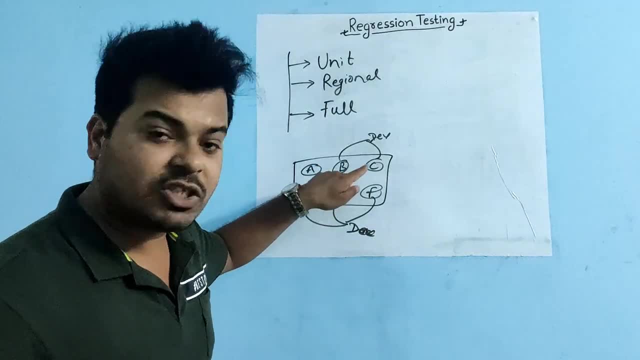 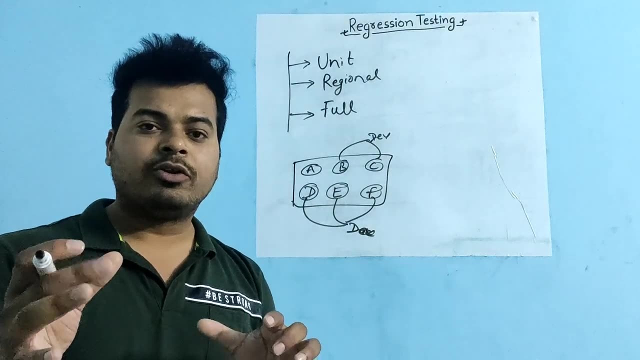 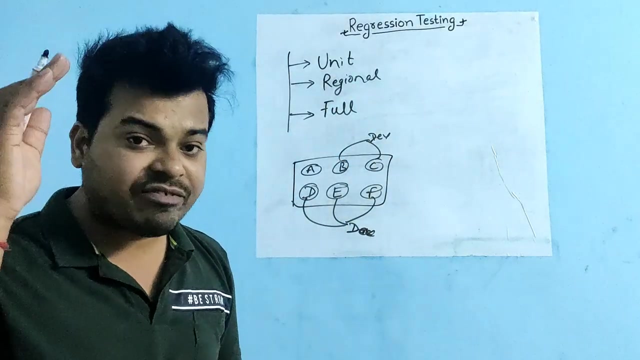 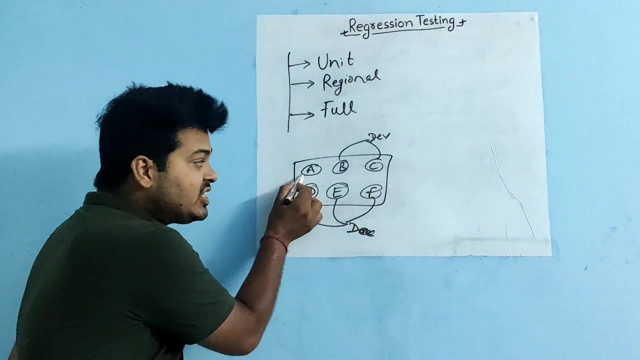 retouching testing, which means not only the modification modules you have to test, but you also have to test the remaining feature of an application. that means, but indirectly, you have to test the whole application, just to make sure that if developer has done some changes in my module, in these modules it is not impacting the unchanged feature. 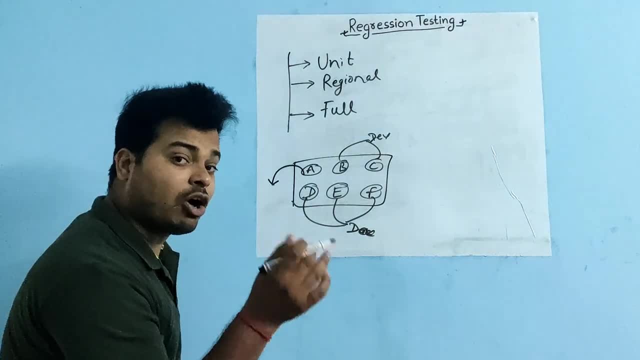 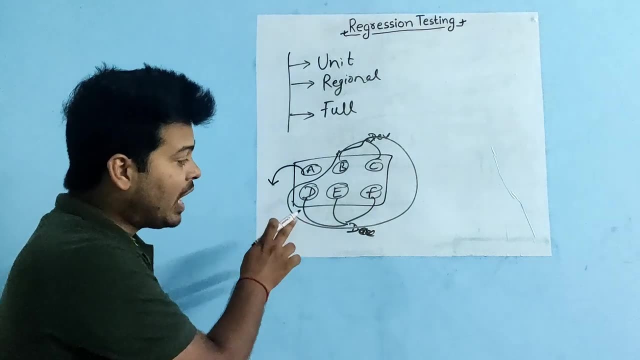 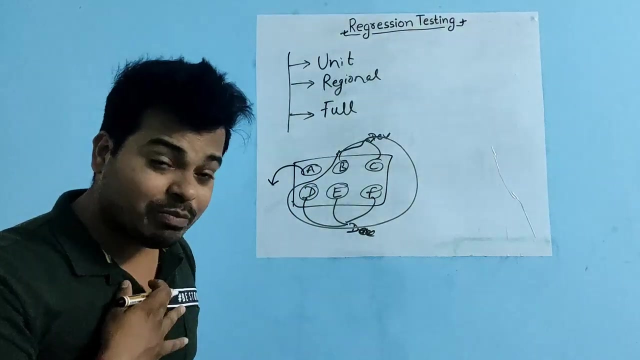 of an application. if my developer has done some changes or modification or fix the defect, they have removed the feature from these five modules. finally, i am going to test all this module, plus all. i'm also going to test my module a, which is untouched, just to make sure that this is not. 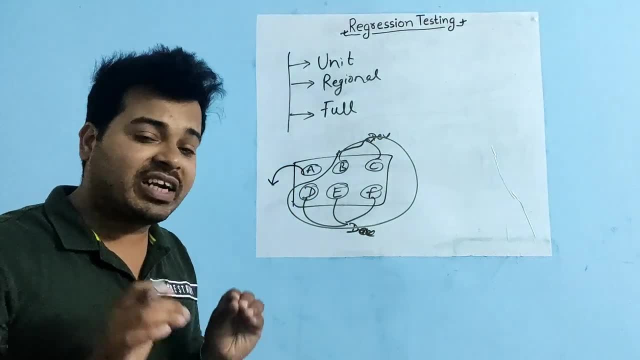 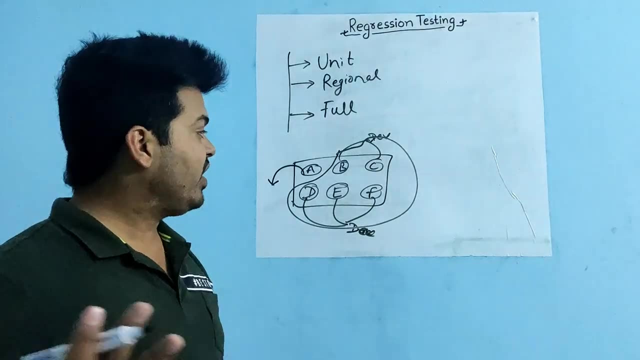 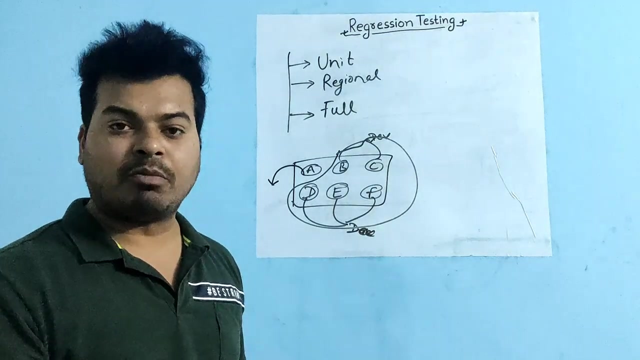 impacted. my module a is working perfectly fine, so this is called as full regression testing. now there are many interview questions which people can ask you, like when we should go for full regression testing, so your answer should be: when developer has done some changes in most of the modules. don't waste time in finding out the impacted areas directly. proceed for. 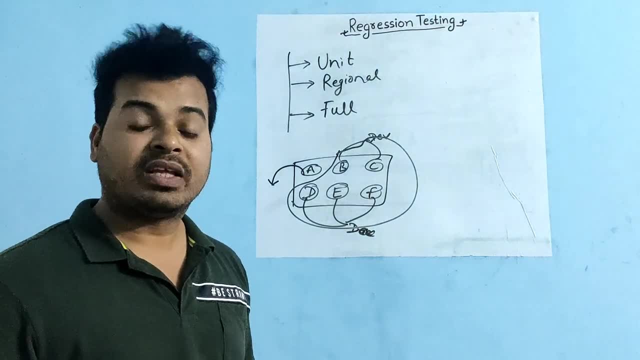 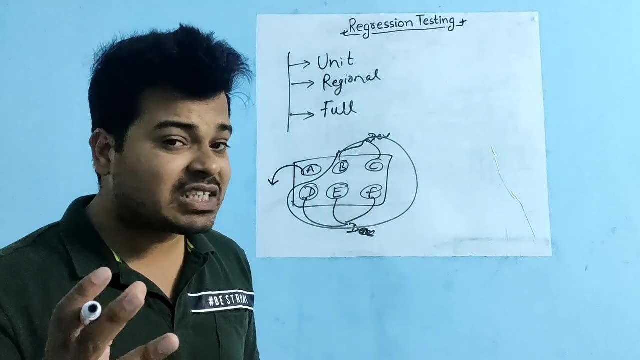 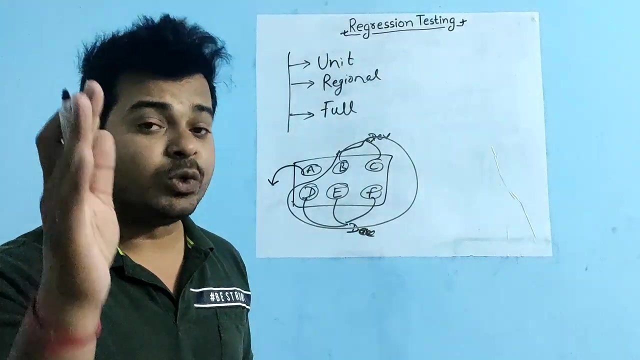 testing. second point is when developer has done some changes in the root of the project. if developer has done some changes in the root of the project, that time it is highly preferable, it is highly advised, to do full regression testing, since my developer has done some changes in the root of. the project. i am not going to take a chance. i don't want my customers to blame me later that this is not covered as a part of your testing. we are finding a bug in the production now. so to avoid those scenarios, if developer has done some changes in the root of the project, we have to do full regression testing. 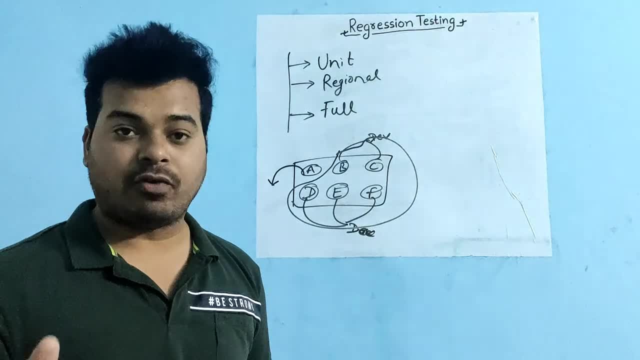 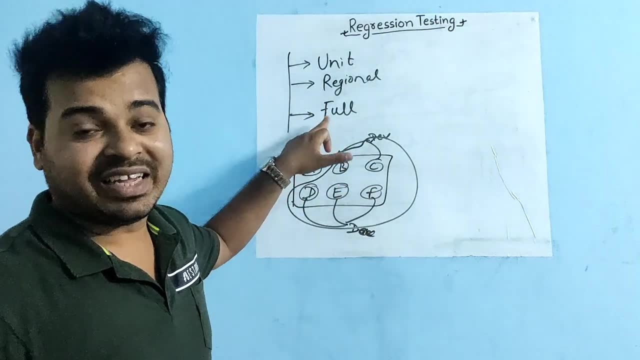 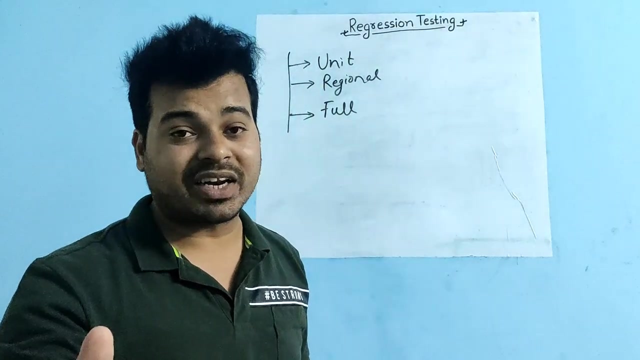 and also third part, when your application platform or your environment itself is changed. that time it is highly advised to do full regression testing. guys, since we are discussing regression testing, i want to tell you, guys, one more thing which no one will tell you is that. so tell you about regression testing. so suppose your sprint is there. your sprint is there for 14 days. 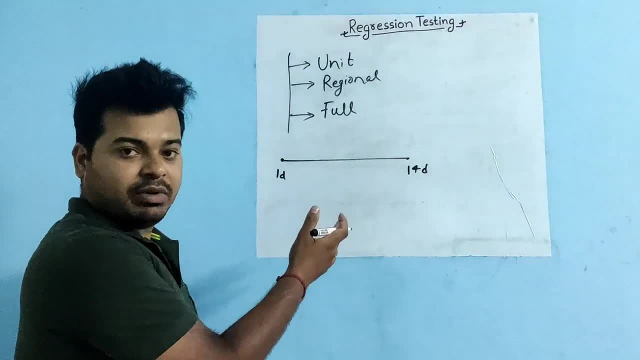 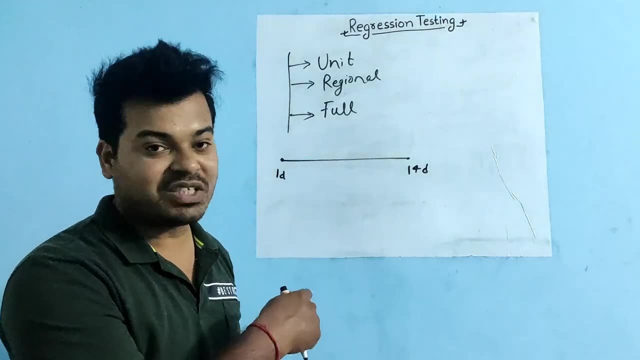 one day, 14 day. that means sprint is nothing, but if you have any doubt regarding what i'm talking- link is there in the description- please watch my agile model video. come to this video. suppose your sprint is there for 14 days. it means you are finally delivering the piece of the software. 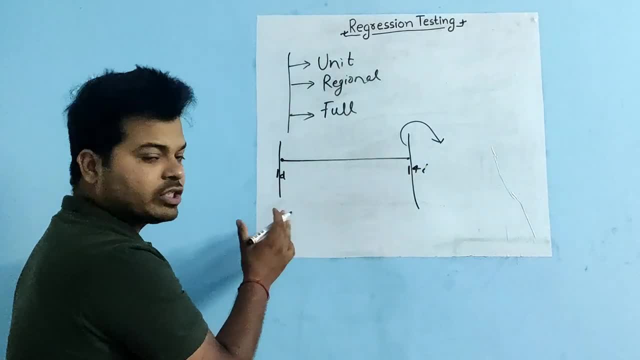 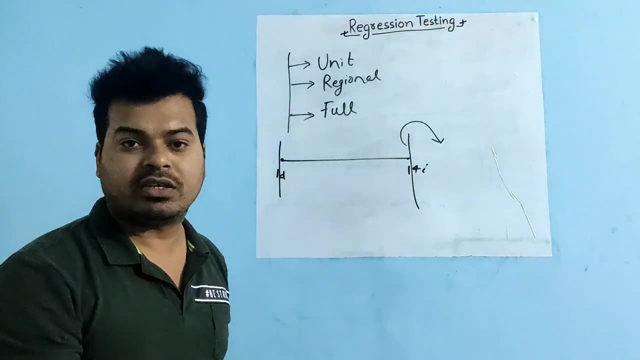 to the customer after 14 days, when your your sprint is having for days. so in the sprint, what you will do, you will. there will be multiple tasks, like some new feature or some modification or some changes in the present feature or dropping of some existing feature. so this: 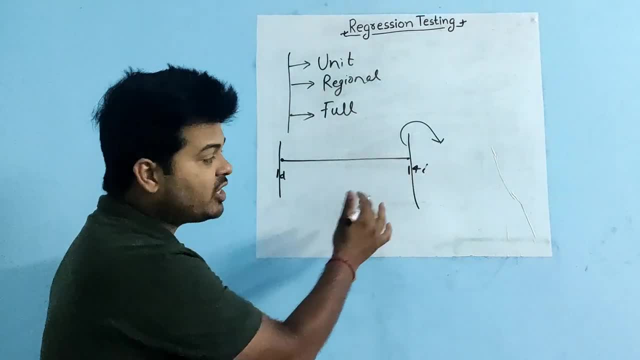 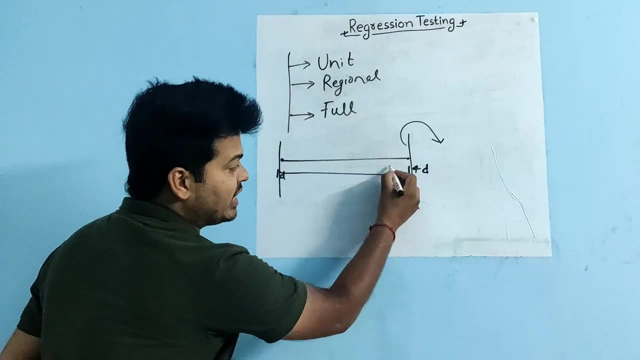 whole task will be there. so if you are having a sprint of 14 day- let's say just an example- different company will have different thing. if you're having a day for first two well days, testers will be involved in testing some new feature testing. they will be involved. 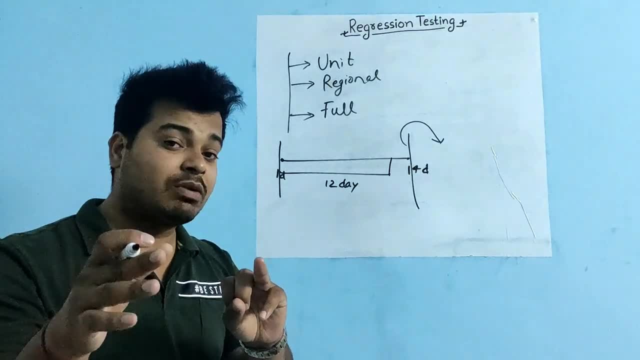 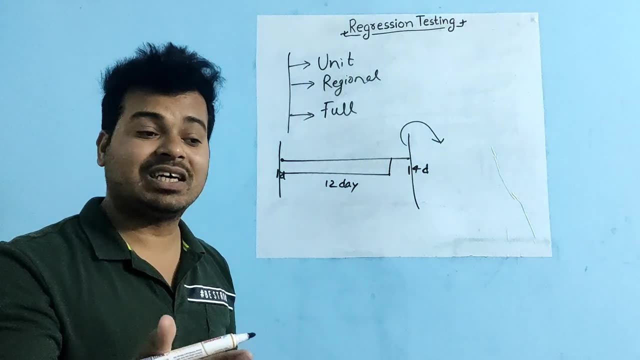 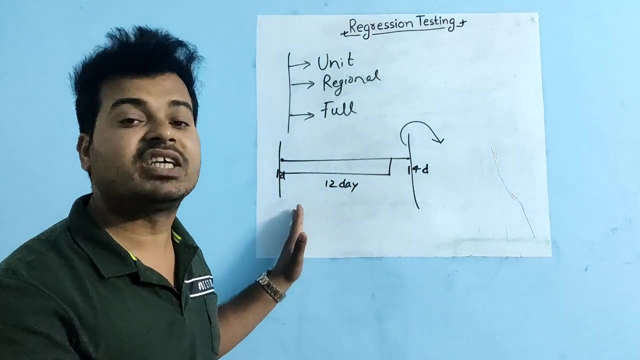 in testing some modification which is done by developers. testers will be involved in testing my modification, which is done in some application, and they will be involved in retesting the fixes. developer has done so. this 12 days you will be completely involved in testing: your feature testing or your retesting, which is that which 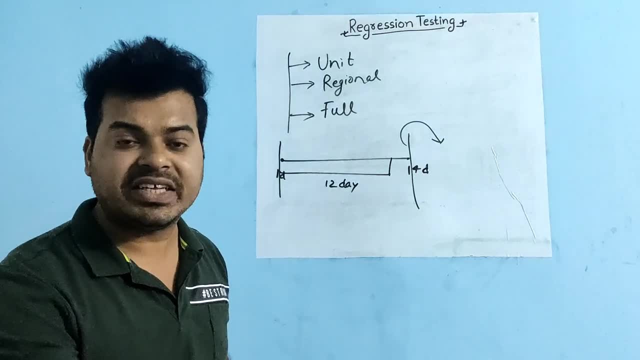 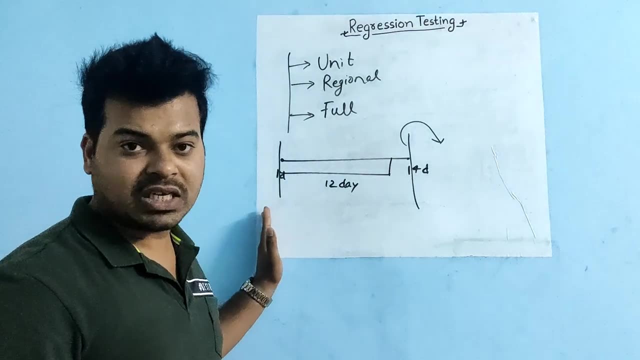 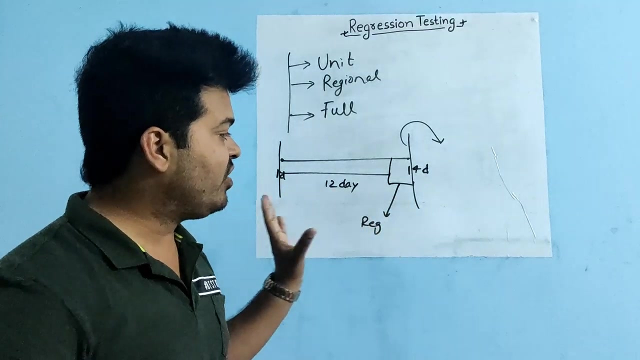 is nothing but testing the bug which you had raised and finite developer has fixed it. now you are testing it. so first 12 days you will be involved in testing all those things. finally, left two days- you will do regression testing because after 14 days we are going to deliver. 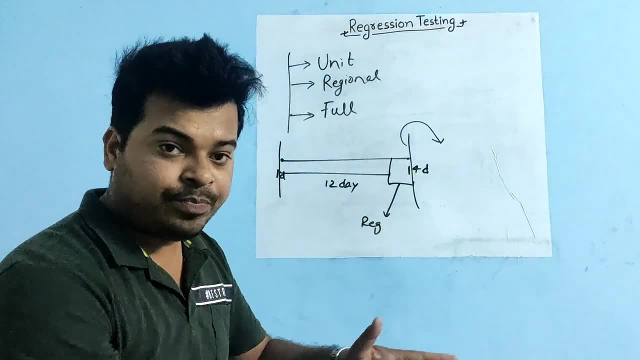 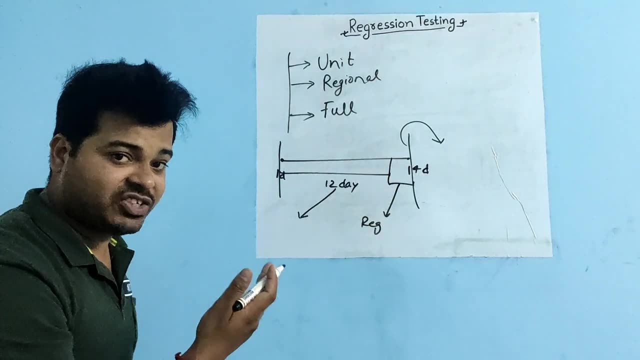 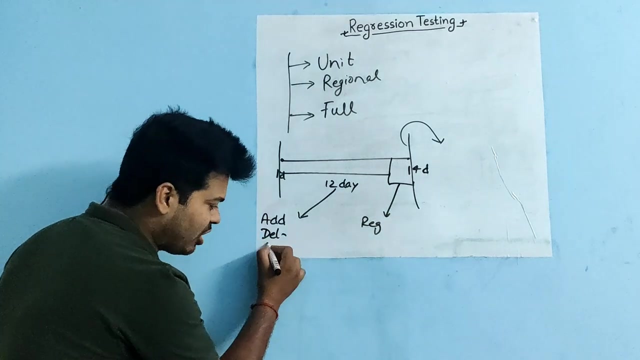 whatever we have done in this 14 days to the customer. we are doing regression testing now because first 12 days we have done lot of changes, changes like we have added some feature, we have deleted some feature, we have done some modification and we have fixed some bugs. so first 12 days, you 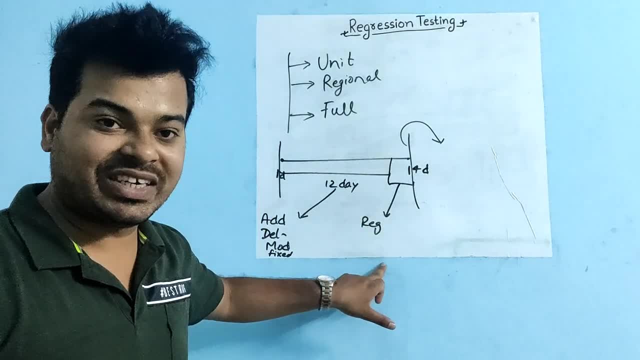 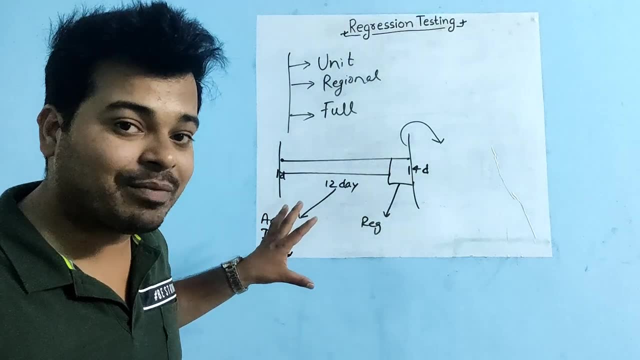 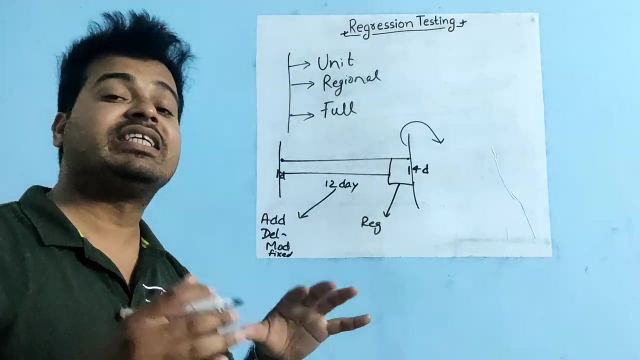 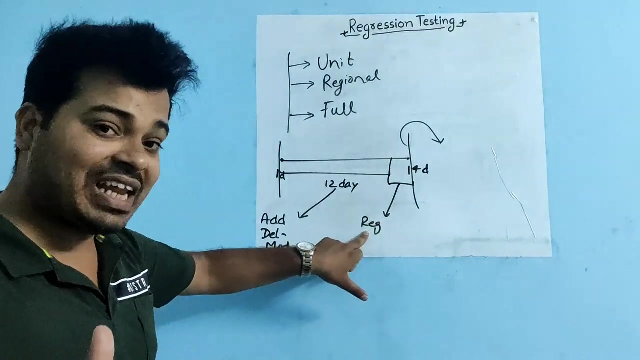 will test all those things last two days. you will do regression testing just to make sure that whatever the changes your developer have done is not impacting the unchanged feature of your application. whatever the changes your developer has done, it is not impacting the whole application. so we do regression testing to make sure that changes like adding a feature, deleting a feature, modification done is that application or fixing the defect is not impacting the unchanged feature, the feature which are not at all touched. that is called as regression testing. so after my 14 days are over, my regression testing is completely done. finally, we are going to deliver the piece of the software to the customer. so this is all. 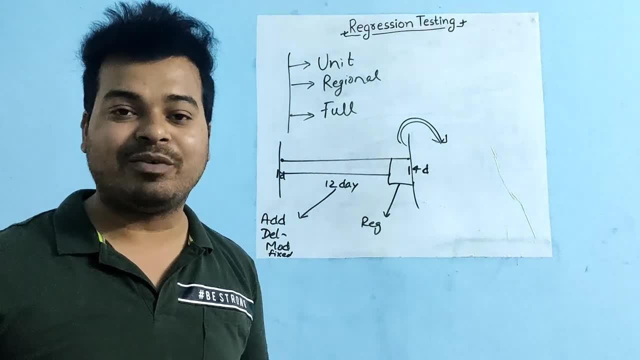 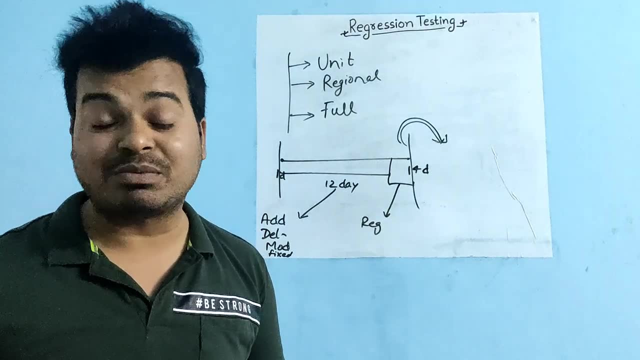 about regression testing. if you have any doubt regarding this video, please list out all your doubt in the comment section. I will be answering. if you want to reach to me personally, I have added my gmail account in the link description. please check it out if you think this video was useful to you guys. 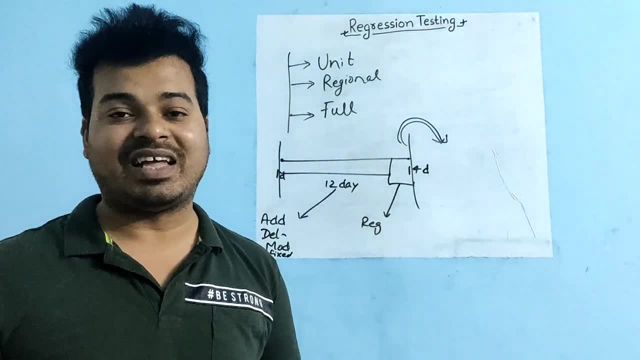 please like this video. subscribe to my channel.